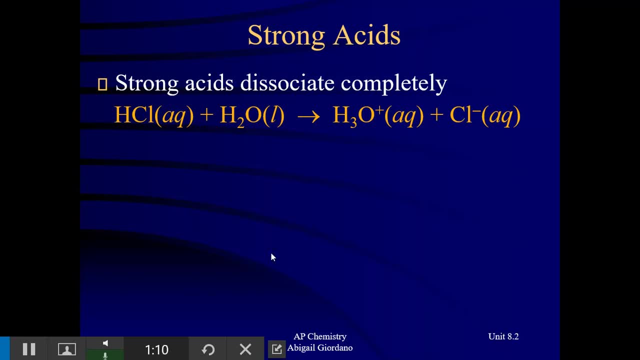 this reaction is essentially going to go to completion, Meaning at the end of the reaction there will be very little, if any, HCl molecules. They are all going to be converted into hydronium and the chloride ion. Now the nice thing is, when we're doing strong acid calculations, these are usually very quick. 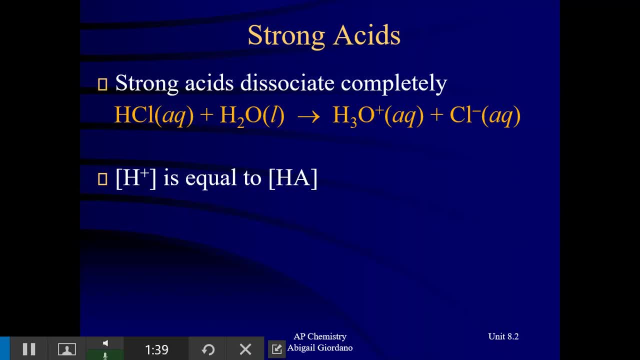 calculations. and the reason is: remember, if you back to our previous lesson, that what you need to determine a pH is the molarity of H+. Guys, remember, H+ is just a shorthand for H3O+, They mean the same thing. 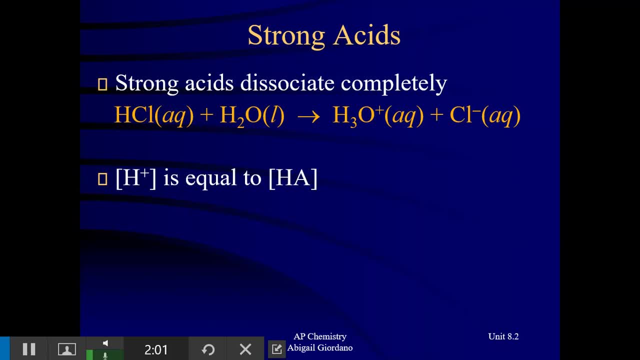 That is very easy to determine the pH of a strong acid because whatever the original molarity of the acid is, That's what I'm representing there with HA- Whatever that original molarity was, because that acid completely dissociates- the molarity will remain the same for the H+. 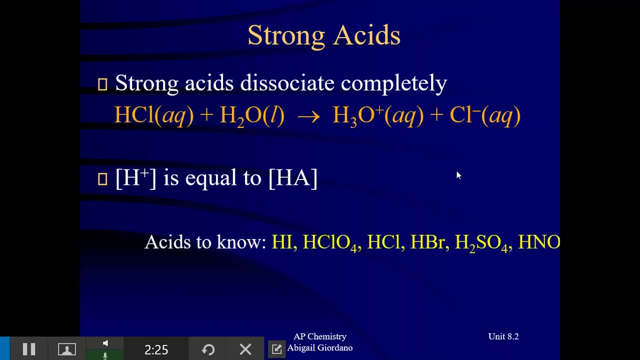 And from there it's very easy to calculate a pH. Now, if you will recall, back to our solubility rules, we had a rule related to acids and it listed these six acids. These are the six strong acids that you need to know. 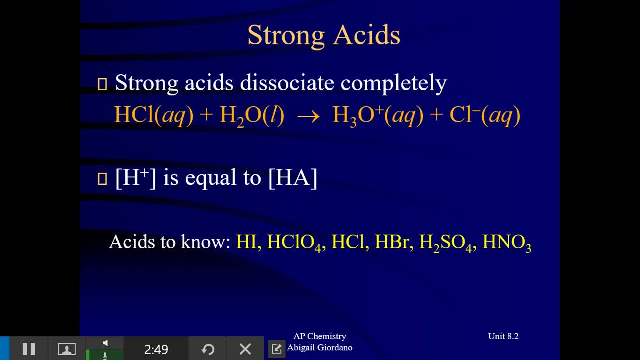 Commit them to memory. ladies and gentlemen, Okay, so these six are the acids that completely dissociate. One thing I do want to just highlight for you is that sulfuric acid. here each hydrogen comes off, one at a time. It is only the first hydrogen coming off being donated. that is a complete dissociation. 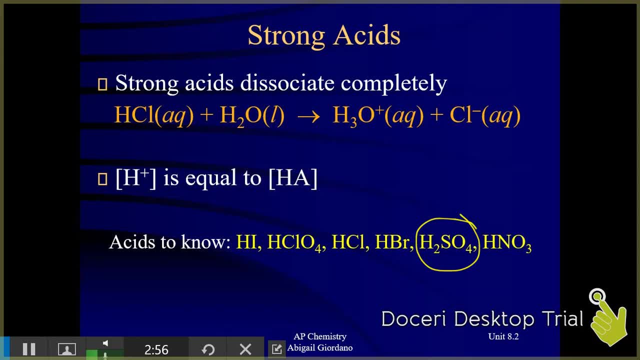 The second, hydrogen, doesn't come off so easily. That makes it a whey Weak acid. we'll talk more about that later. Okay, and I have a little memory trick here to help you commit these six strong acids to memory. All right, and the phrase is: imagine a perfectly clear, breezy summer night. 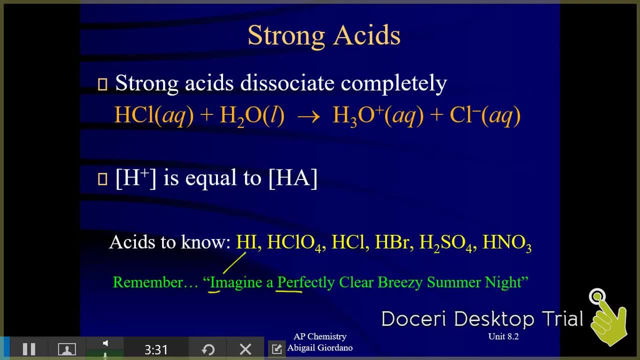 I imagine hydroiodic, Perfectly purr, perchloric Clear, hydrochloric Breezy, hydrobromic, Sulfuric summer sulfuric Night nitric. It is absolutely imperative, ladies and gentlemen, that you commit these acids to memory. 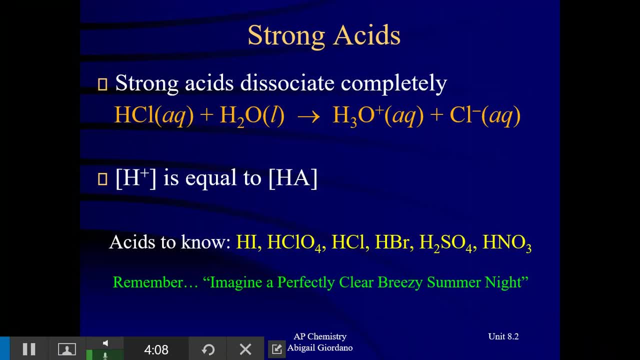 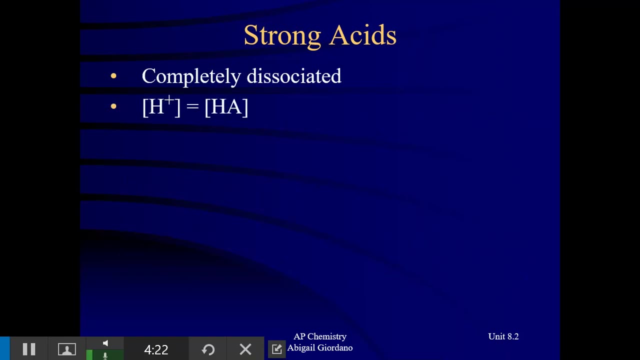 So these are the six strong. Anything that fall, any acid that is not in that list, must be a weak acid, will not completely dissociate, and we're going to talk more about weak acids in a later lesson. So, as we said, they completely dissociate. 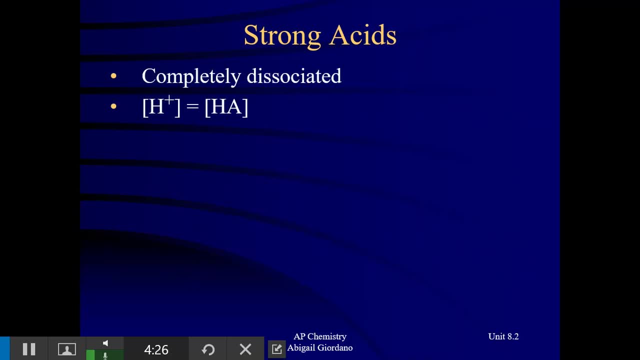 The math is usually very quick, because the molarity of the acid as a whole is also going to be the molarity of the H+. because of that complete dissociation In a strong acid solution, the molarity of OH- is going to be very, very small. 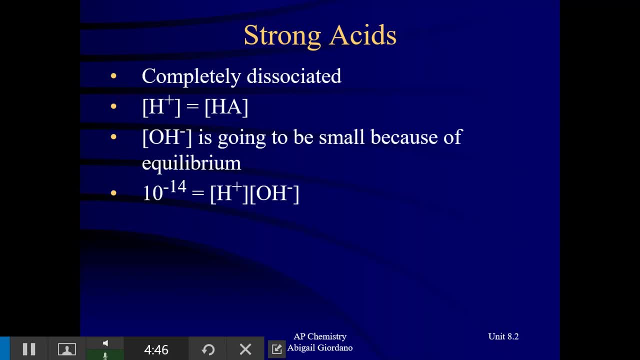 Okay, and think about it. Okay, this is a. this is an equation we looked at in our last class. This is an equation we looked at in our last class. Okay, and think about it. This is a. this is an equation we looked at in our last class. 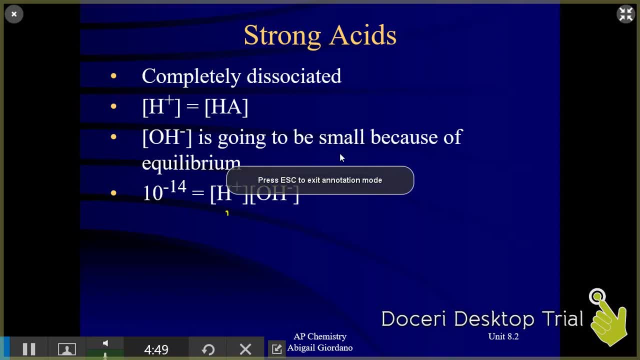 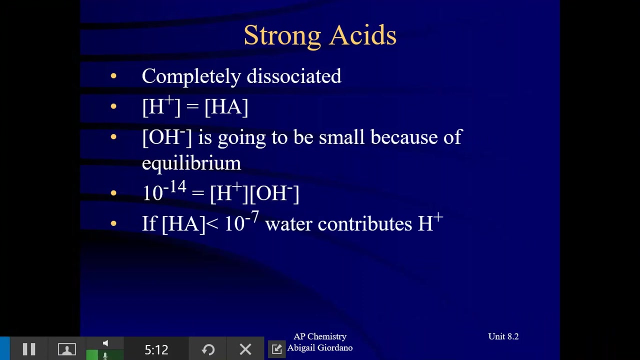 looked at in our last lesson. if this molarity is relatively high, it's a relatively large number. that means the OH minus must be very, very small because of that relationship. Okay, and I'm going to come back and address that bullet in just a second. 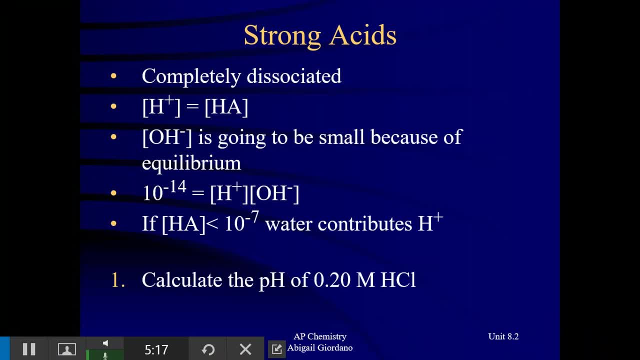 Okay, so let's just look at a very quick little calculation here. It says: calculate the pH of a 0.2 molar solution of HCl Immediately. I recognize, okay, HCl. that is one of my six strong acids. 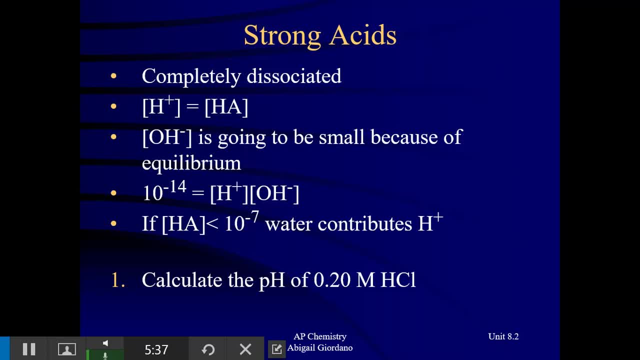 And so, because that is the case, I can assume this- that the H plus concentration is also 0.20 molar. Again, because of that complete dissociation, let's remember what the formula is to calculate pH. Alright, if we take the negative log of 0.20, let's round it to two significant figures. 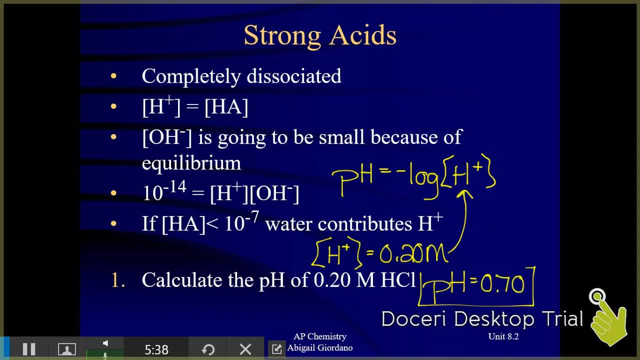 That gives me this. this pH, Okay, and that should make sense to you. Okay, that's a very low pH and it should be. This is a strong acid. Okay, strong acids typically have very low, very acidic pHs. 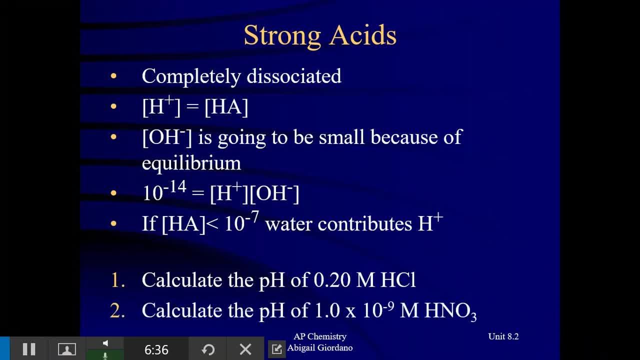 Okay, look at this second one. Same question: different molarity and different acid. This is nitric acid, which is one of my six. This is nitric acid, which is one of my six strong. Okay, now, if you just kind of went into auto-pilot mode and you said, okay, there's the molarity of the acid. 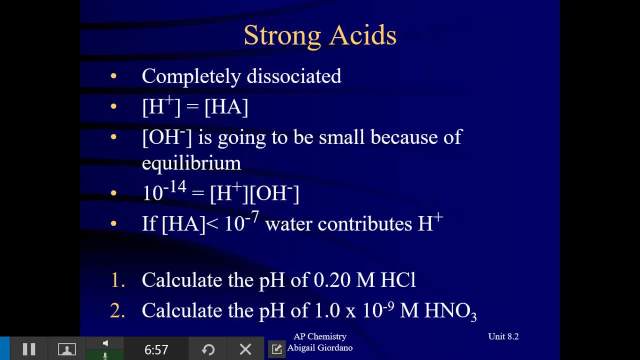 That's going to be the molarity of the H plus ion as well. Hmm, let me take the negative log of that number. Ladies and gentlemen, that's going to give you a pH of nine, And I want you to think about that number for a second. 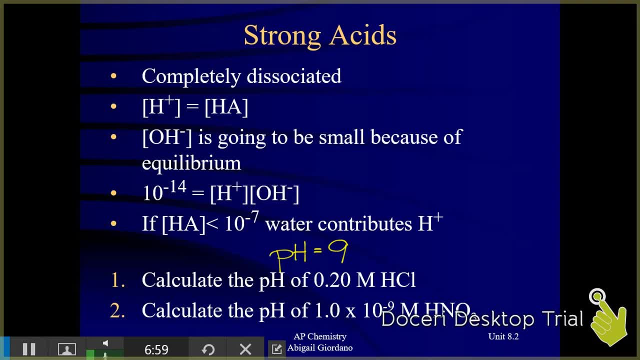 What kind of sense does that make? This is a strong acid. How could it possibly have a pH in the basic range? That doesn't make sense, And that's because that's not correct. Okay, look at this bullet now When you're dealing with this. and, by the way, guys, this applies to strong acids only. 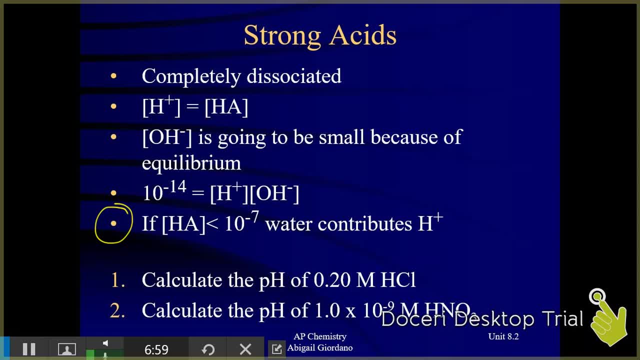 If the molarity of your strong acid is so dilute- how dilute? Well, less than 10 to the negative seventh. That means that it is so dilute that water is in fact the dominant acid in that scenario. Okay, that means water is actually donating away more H plus ions than this very dilute strong acid. 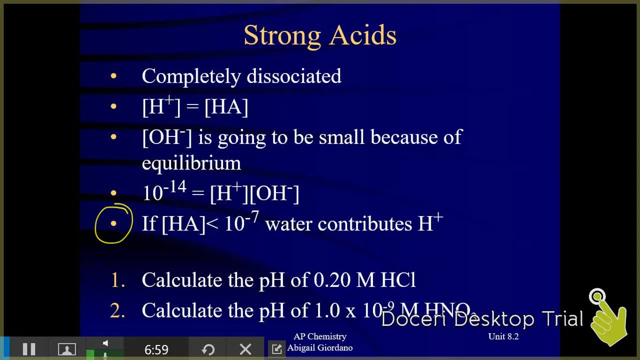 And guess what, guys? If water is your dominant acid, guess what the pH is. The pH is equal to 7.00.. Okay, Does this situation come up frequently? No, it doesn't Okay, But it comes up on occasion. 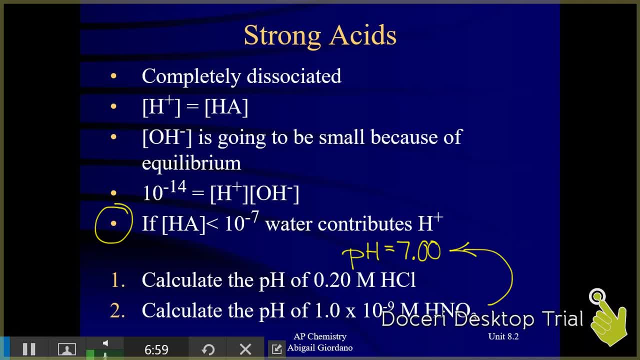 And again, it applies to strong acids only If the molarity of your strong acid is less than 10 to the negative seventh, it is so dilute that water is in fact the dominant acid And you'll get a pH of 7.00.. 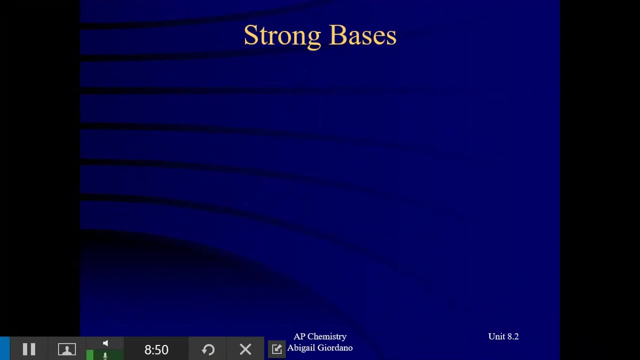 Okay, How about strong bases? Well, guess what The word strong means the same thing. Okay, It's used in the same sense. It is meaning complete dissociation. The only difference here is we're not getting a hydronium or hydrogen ion on the product side. 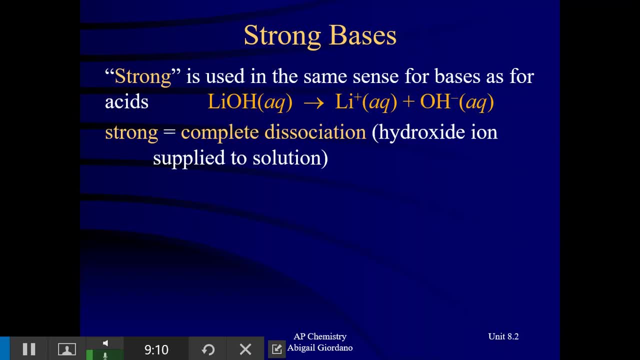 This time we're getting a hydroxide ion. I made you memorize your strong acids. Ladies and gentlemen, you need to memorize your strong bases as well. Okay, What do I mean by group one hydroxides? That means any metal, any group one alkali metal joined to hydroxide. 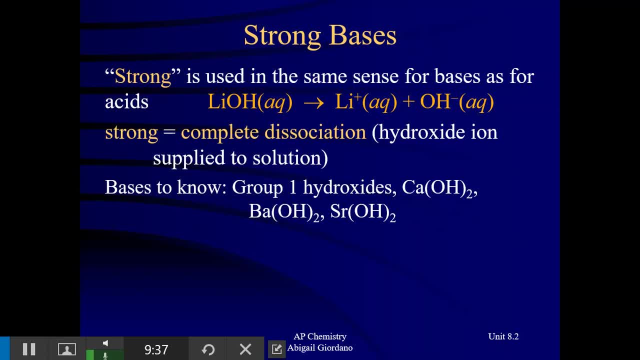 Lithium hydroxide, Potassium hydroxide. Those are all strong bases. From group two. you have three of them: Calcium, barium and strontium hydroxide. Okay, I always hear my students, you know, saying: okay, which ones are the strong bases? 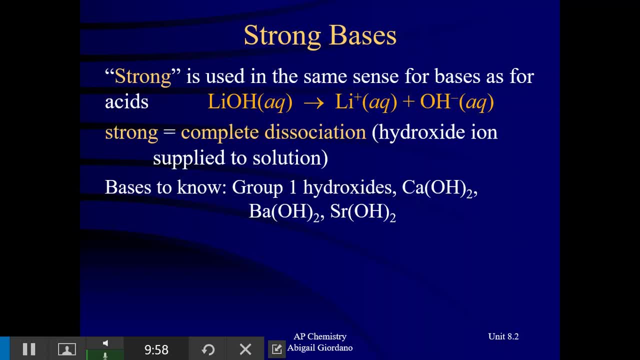 And I kept hearing them years ago saying cabasser, Cabasser And I was like what are they saying, Cabasser? Calcium barium, strong bases, Calcium barium, strontium. It was their funny little way of remembering those strong bases. 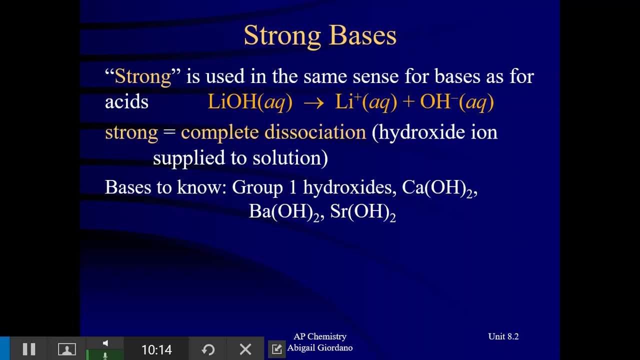 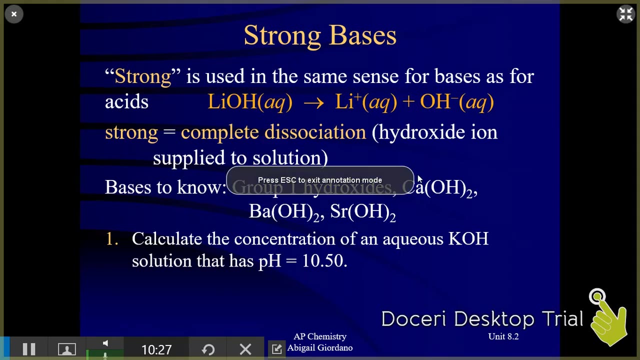 Just don't forget, it's also group one as well. So all of those bases completely ionize when they're in an aqueous solution. Okay, So let's just work one together. All right, Let's see how we do, Okay. 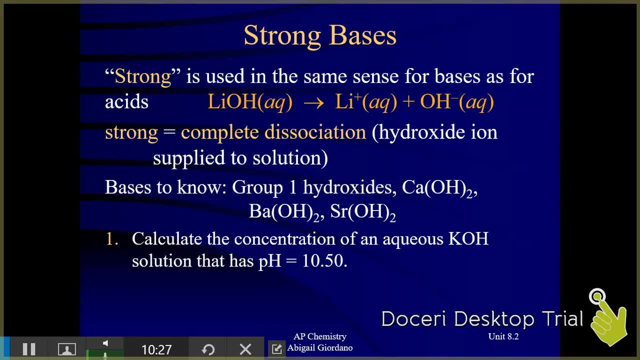 It says: calculate the concentration of an aqueous KOH solution that has a pH Of 10.5.. Well, right off the bat, I recognize. Okay, This is one of my strong bases. Okay, So I'm going to write. 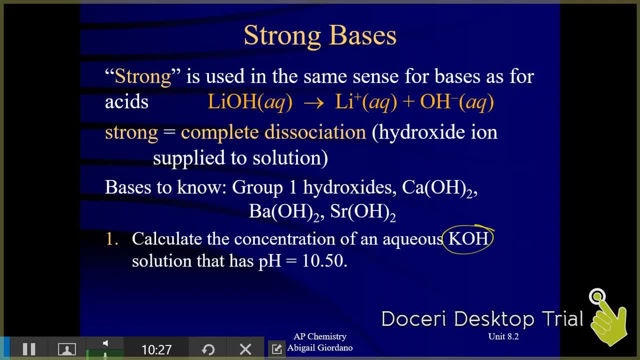 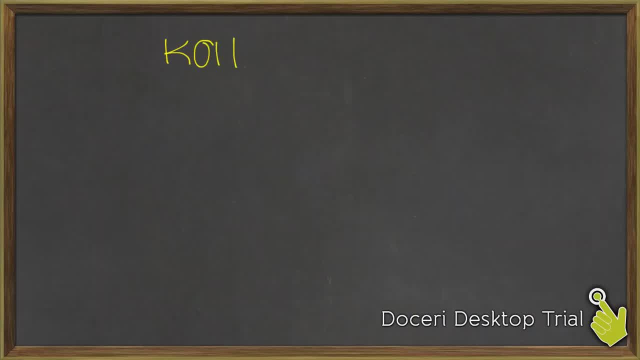 In fact, you know what I'll do. I'm going to open up a new screen, Okay, So let's think about the formula for KOH And how that would completely dissociate, Completely dissociate. Okay, They told us the pH. 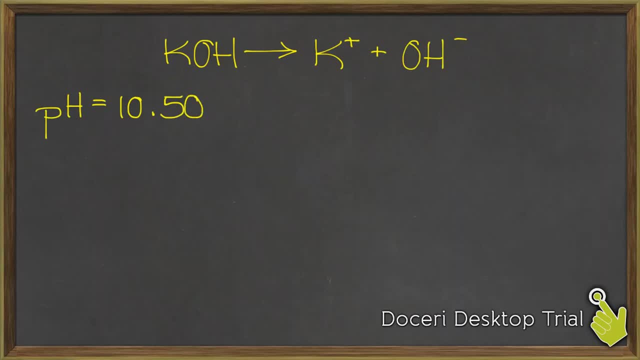 Was 10.50.. And that makes sense. It's a base, Okay, Well, let's turn that into a pOH. Okay, 14 minus 10.5.. There's my pOH, And let's think This is what I'm trying to find the molarity of. 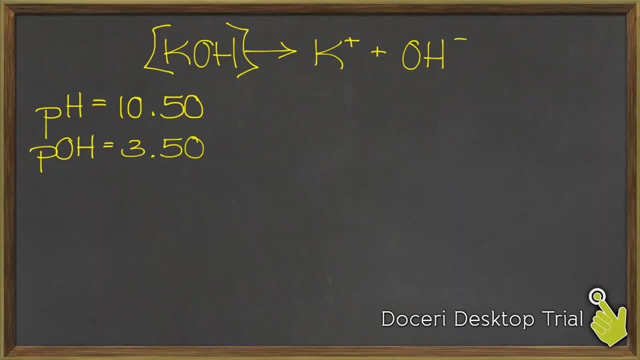 Let's think about what we could do next. How about if we use this equation? Okay, I'm going to plug in my pOH And to invert a log. We do 10 to the power of negative 3.5. And I get this. 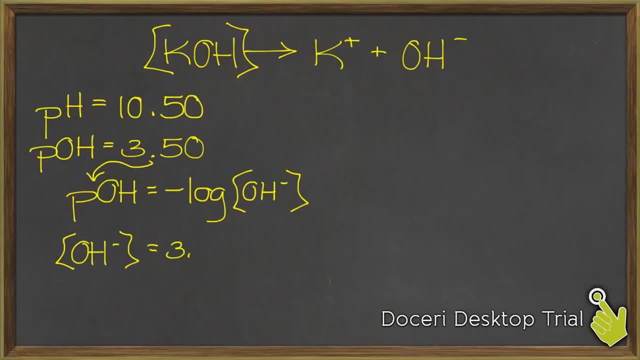 I'm going to round my answer to two significant figures. Okay, Now, that's not quite the final answer. That is, the molarity of OH minus. This problem actually asked us to find the molarity of the pOH And the molarity of the base as a whole. 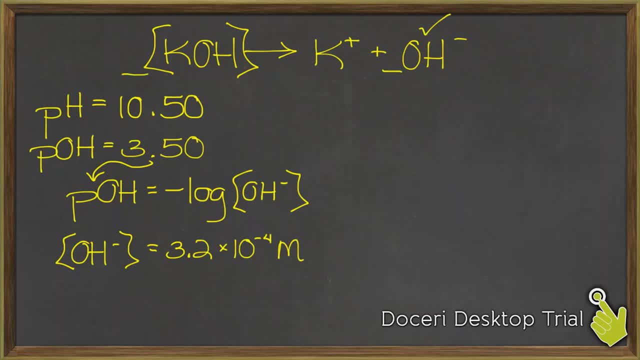 But, ladies and gentlemen, do you recognize that these two things are in a one-to-one ratio? So guess what? It'll be the same number. Now, is that the case for all bases? No, it isn't, And we don't really have to deal with this with acids so much. 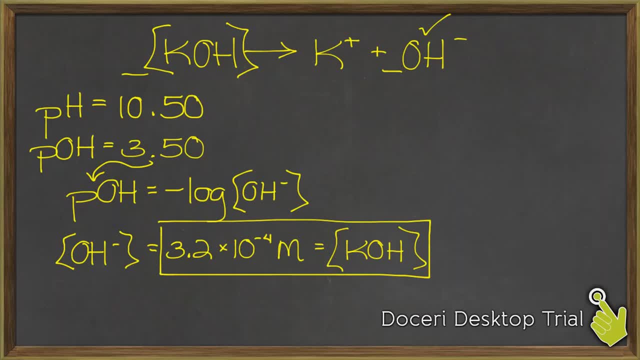 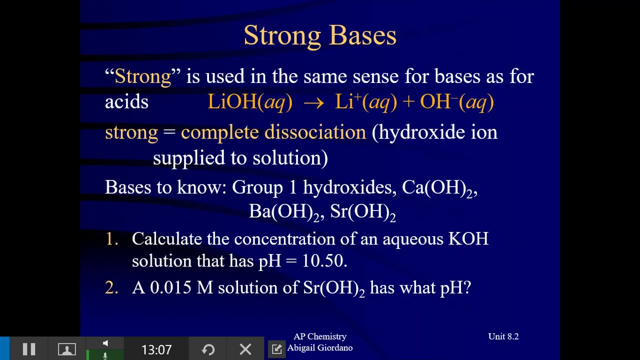 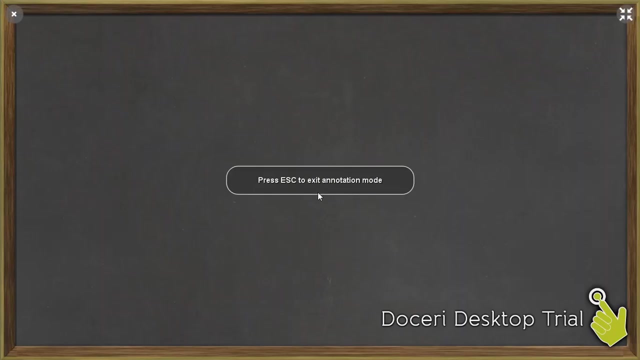 But three of our strong bases come from groups Two: hydroxides. So look at this problem. It says a 0.015 molar solution of strontium hydroxide has what pH? Okay, Well, let's start off just like we did with the other one. 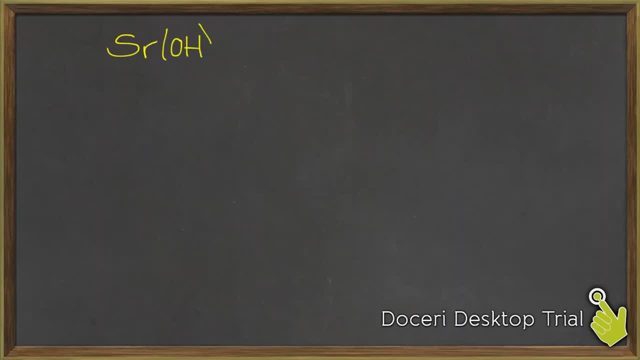 Let's write out the equation for how this base is going to react. It's going to dissociate. There's two hydroxides in there. Okay, Got to make sure you have a balanced equation. And let me come back here. What did they give us? 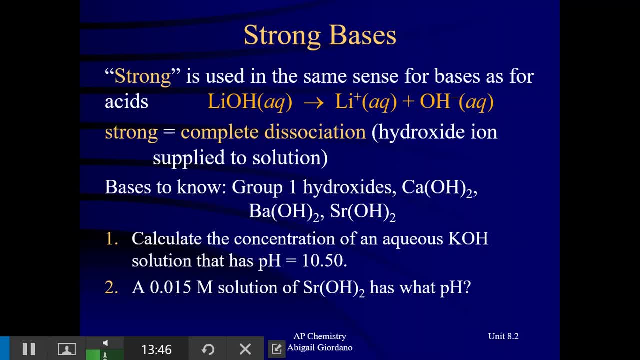 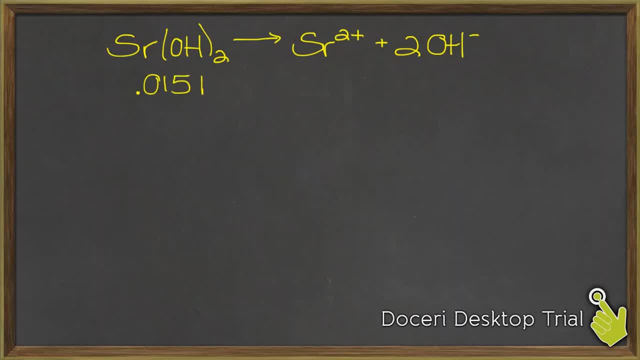 They said that the solution, the molarity of SROH2 is 0.015.. Okay, Well, based on the stoichiometry, ladies and gentlemen, based on the fact that these are in a 1 to 2 ratio, 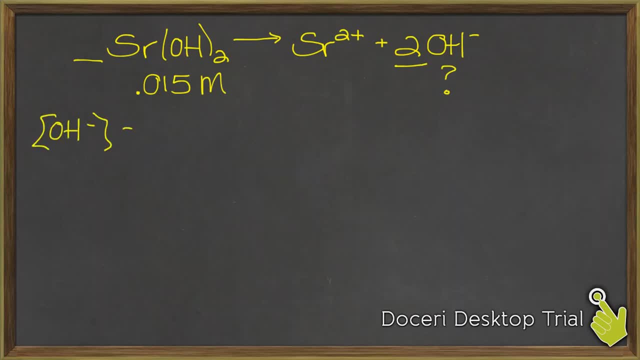 hopefully you can recognize that the OH- concentration is going to be double: 0.015.. It will be 0.030.. And think about where you can go from there. Can't you now find the pOH? Let's see what that gives us. 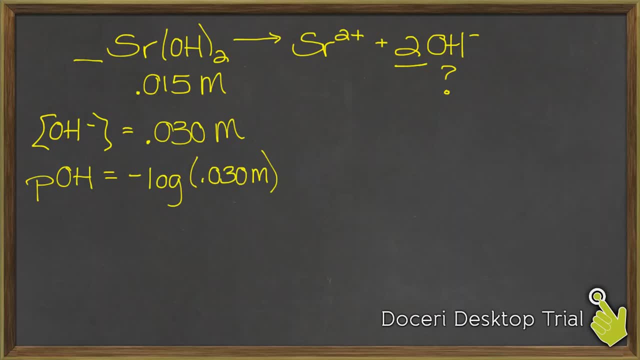 Negative log of 0.030.. Okay, So my pOH is 1.52.. The problem wanted us to calculate the pH. So if I do 14 minus that pOH, final answer, And I want you guys to start getting in the habit of asking yourself. 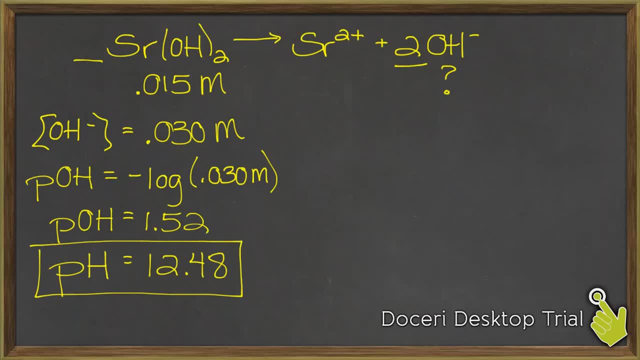 does my answer make sense? You're going to get so sick of hearing me ask you that. Think about the situation here. We have a strong base. Does a pH of 12.48, does that make sense? Absolutely it does. That pH is in the basic range and it's kind of high in the basic range. 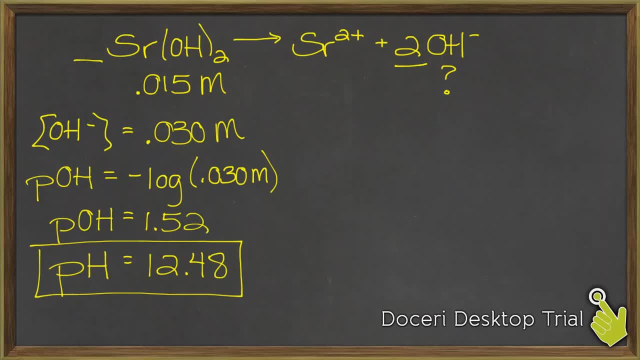 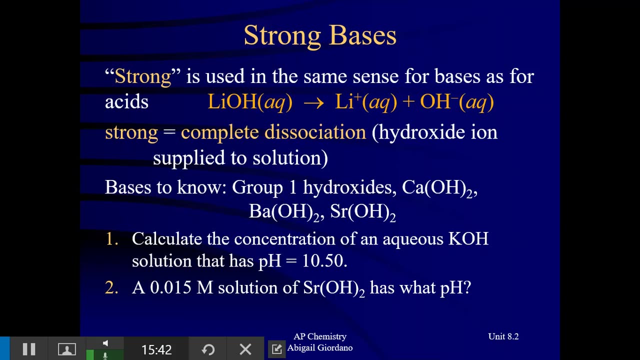 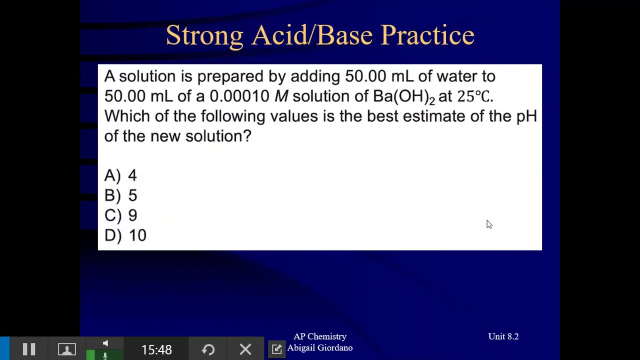 And that makes sense for a strong base. So in general guys, these strong acid and base calculations are usually pretty quick. So let's look at some practice AP kinds of questions. I'm going to work this one with you and then I'm going to give you a chance to do some on your own. 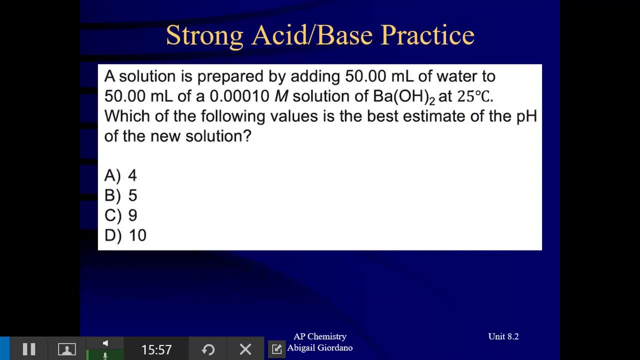 All right. This one says a solution is prepared by adding 50 milliliters of water to 50 milliliters of 0.0001 molar solution of barium hydroxide at 25 degrees. Which of the following values is the best estimate of the pH of this new solution? 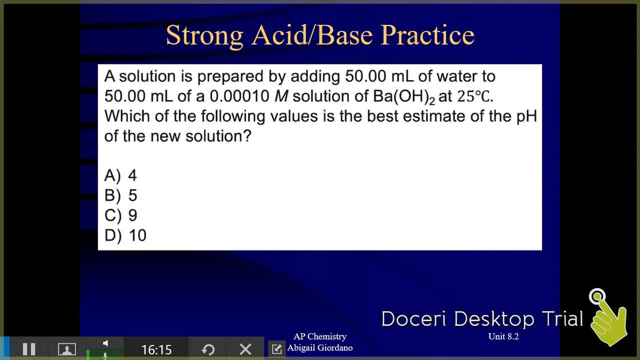 And it's multiple choice. So let's imagine this is a real AP exam question where you do not have a calculator. Guys, it's a basic solution. I would hope that you would immediately be able to eliminate answer choices A and B, because those are acidic pHs. 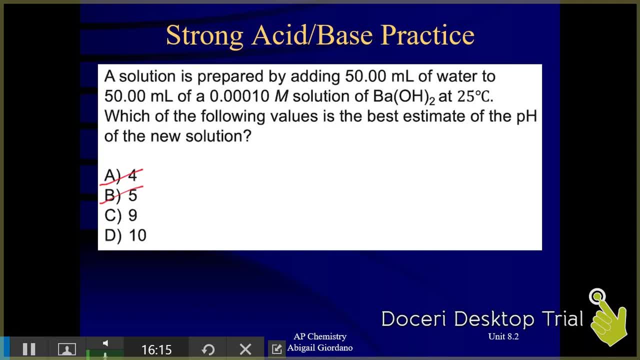 Okay, Those don't make sense. We could at least narrow it down between C and D, But let's talk it out. So what's going on here? I have a sample of a barium hydroxide solution And what am I doing to it? 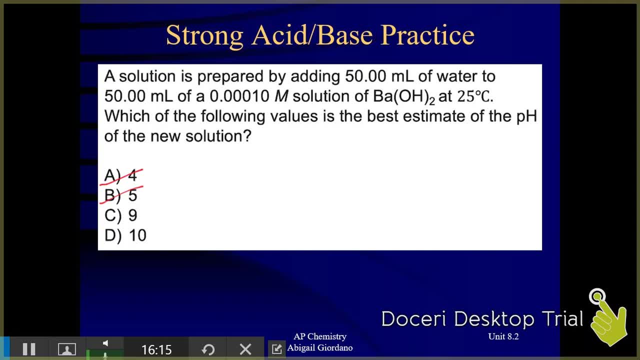 I'm just diluting it Which, ladies and gentlemen, if you remember, this is the dilution equation: M1V1 equals M2V2.. Okay, This barium hydroxide, Before it was diluted, There's M1.. 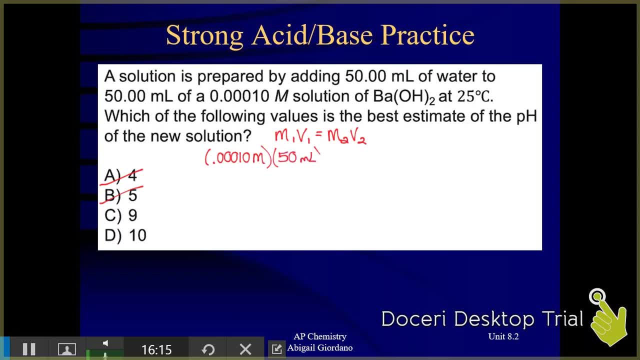 This was before it was diluted. After it's diluted, I don't know what this molarity is, That's what we're going to find out. But it's total volume now. because I added 50 milliliters of water, The total volume there is 100.. 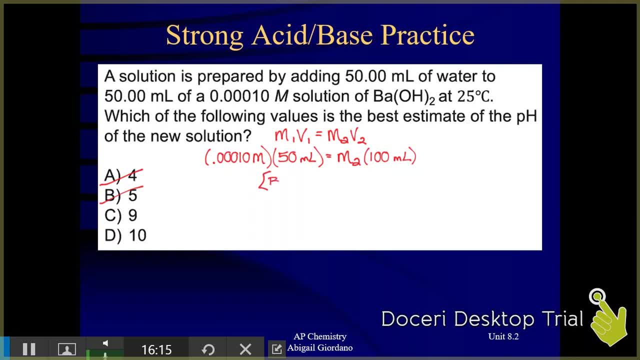 Okay, So this is the molarity of My barium hydroxide solution And I get this. Okay. Now remember guys, when you're finding a pH, You need to know the pOH, or you need to know the H plus concentration or the OH minus concentration to help get you there. 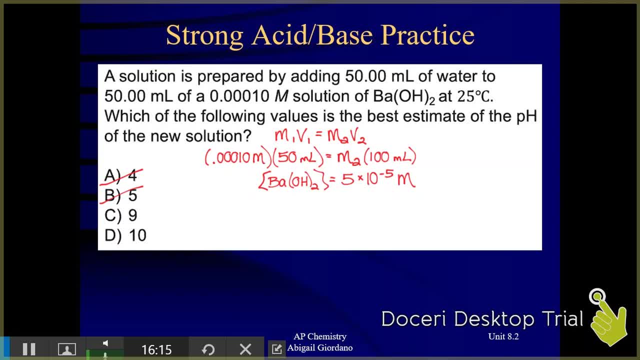 At the moment. this is not A hydroxide ion concentration. This is the concentration of the whole Compound. Think about The balanced equation when this base dissociates. Oops, Okay, We just solved For the molarity of this guy. 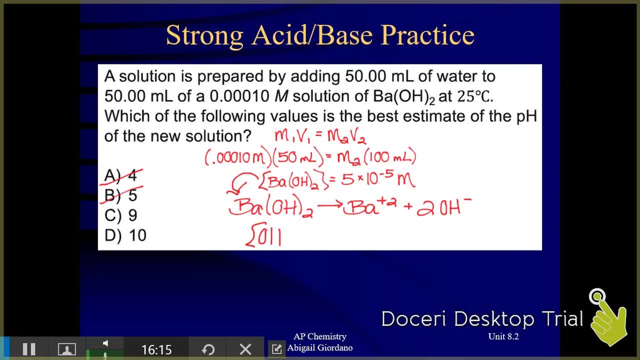 So what is going to be the molarity of OH minus? It's going to be double That number, Which gives me this All right. What would be the logical next step? to find, Probably the pOH. Okay, Now, if you've been using a calculator, 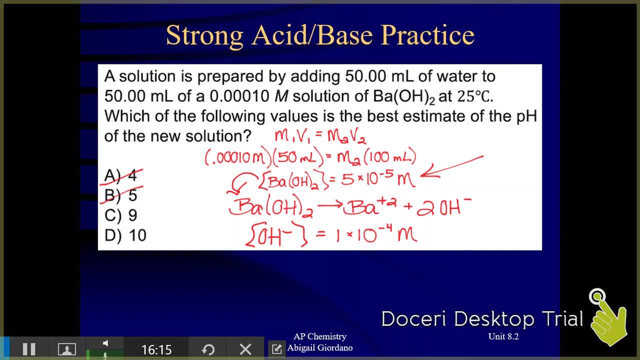 As you've been doing this with me, Put it down. Remember, we talked about estimating pHs and pOHs. To find this pOH, If I take the negative log Of this hydroxide concentration, The pOH is going to be equal to exactly. 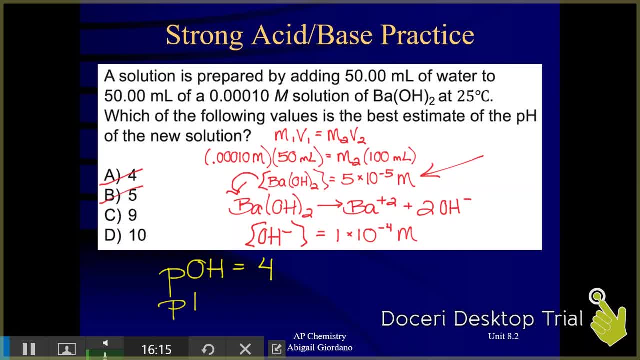 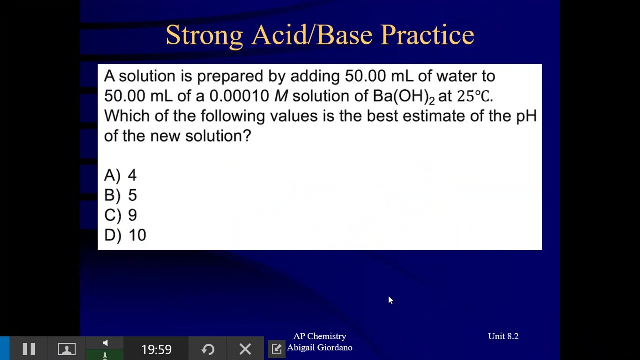 Four, And then from here it's easy: Fourteen minus four, The pH is ten, So D is my answer. Okay, That is something the AP exam would expect you to be able to do without a calculator. All right, So here's another multiple choice question. 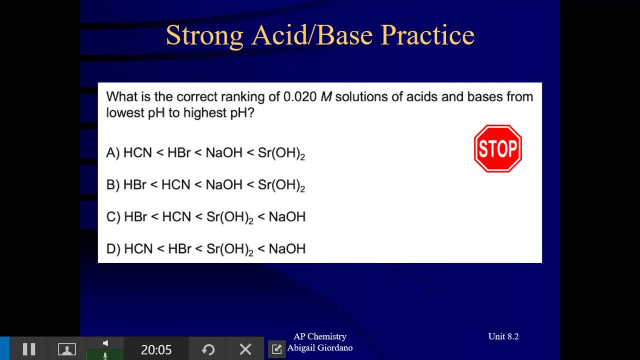 This one is addressing sort of a different situation, But I want you to pause the video. See if you can solve this one. See if you can solve this one on your own. Okay, So it says that we have .02 molar solutions. 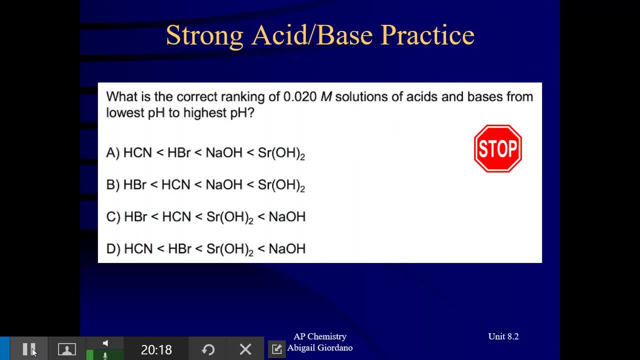 Of all these acids and bases, And we are supposed to rank them From lowest pH To highest pH. Let me say that to you in another way: Most acidic To most basic. Okay, So let's look at these four species that we're dealing with. 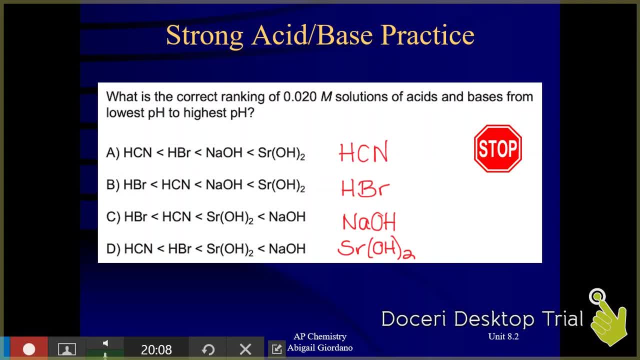 And let's decide. you know what are these things? Well, HCN is an acid. It is not one of my six strong, So this is a weak acid. HBr is one of the six strong, So I'm going to write strong. 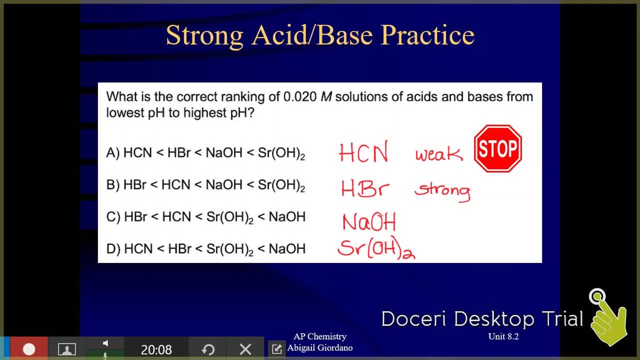 Okay. So before I go any further, Based on the fact that HBr is strong And HCN is weak, An equal molar solution of those two acids. The strong acid should be more acidic. It's going to have a lower pH. 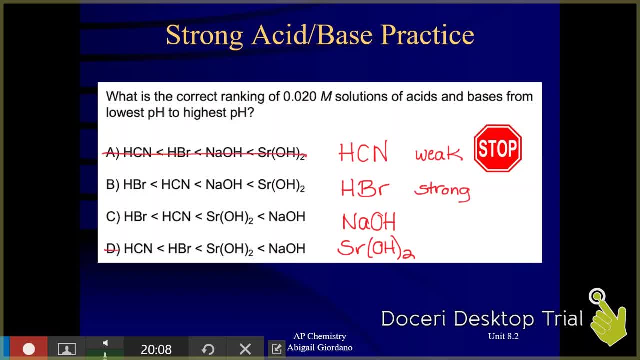 So right away I'm going to eliminate A and D, Because that weak acid is not going to be the most acidic. Okay, So now it's down between B and C. Now this is a little tricky, Because both of the bases here 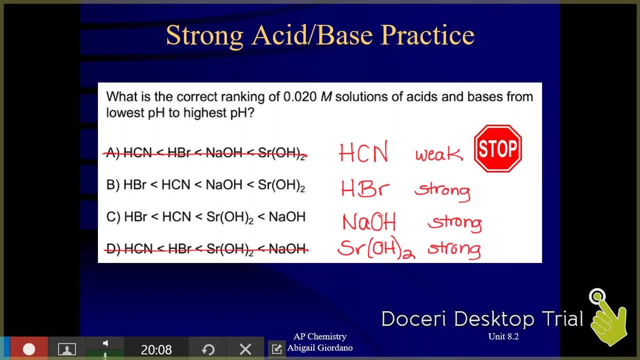 Both of the bases are strong. But come back up here We have 0.02 molar of all of these solutions And both of these bases, But the strontium hydroxide- Remember, it's got two hydroxide in there. 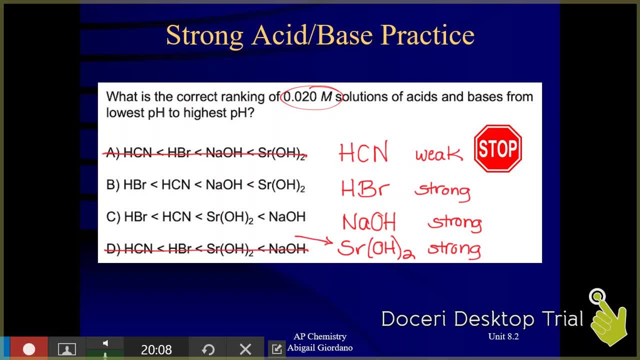 When it dissociates, It's going to have 0.04 molar For its OH minus concentration. Strontium hydroxide is going to have a higher molarity of hydroxide And that's going to determine the pOH. 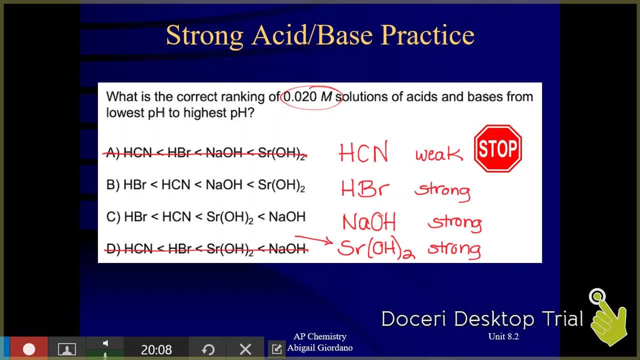 And thus the pH. So because strontium hydroxide is going to be providing Double the amount of hydroxide That's going to cause that solution to be the most basic. So B is my answer, Okay, So sometimes you'll have conceptual questions like that. 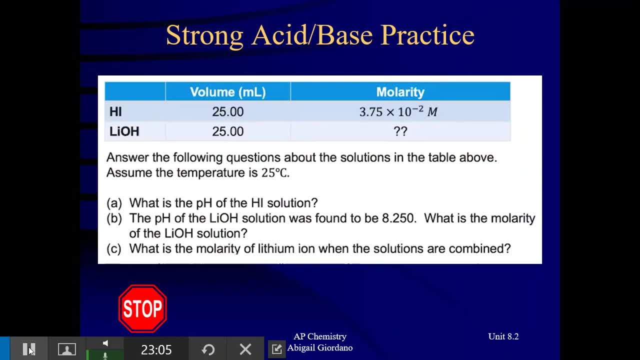 Okay, So here's one more question. This kind of pulls a lot of the topics together. This is more like what you would see in a free response situation, So pause the video, See how you do with it. Okay, So let's look at the situation here. 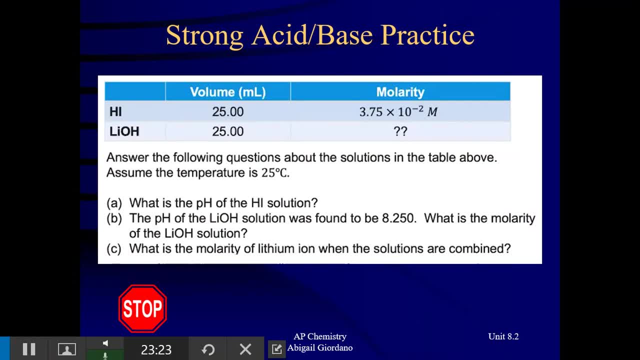 We've got An acid HI, One of our strong ones. They give us a volume, They give us a molarity. We're given LIOH, One of our strong bases. We're given the volume, But we don't know the molarity. 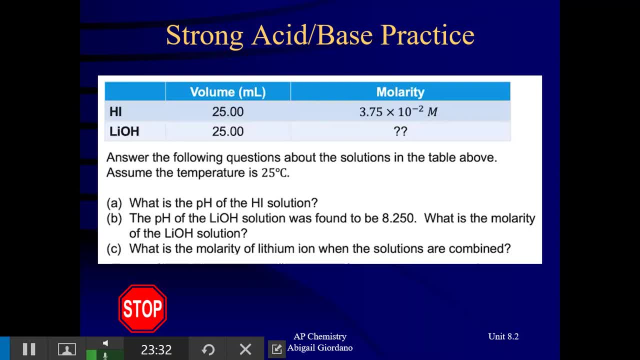 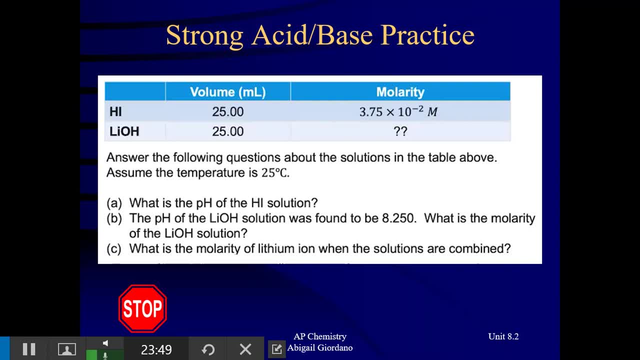 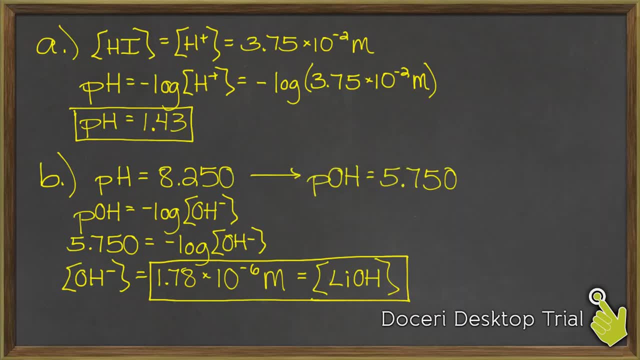 Hopefully Did this pretty easily. We're given the molarity Of The acid itself, That strong acid. So if you look at what I've got for letter A, Because it's strong, I know that the molarity Of the acid itself. 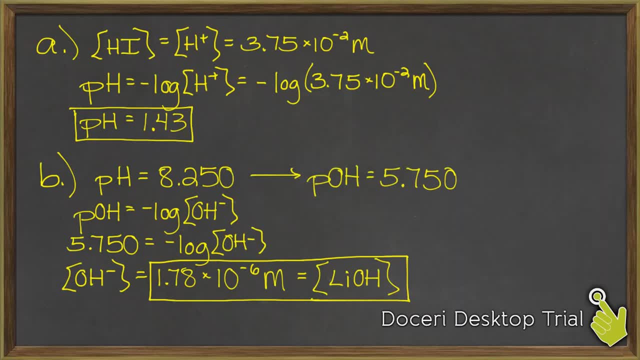 Is going to be equal to the molarity Of H+, Which I can then just substitute into my pH. equals negative log of H" Equation And I get a pH of 1.43.. Asking for LH+ yourself, does it make sense? It does. It's a strong acid. It should have a low pH. 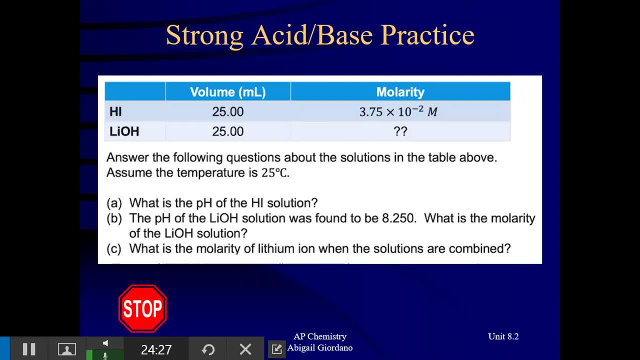 Okay, let's look at part B. It says the pH of the LiOH solution was found to be 8.250.. Makes sense. It's basic: What is the molarity of the LiOH? This is basically just going backwards. So for letter B, we're told the pH, The first. 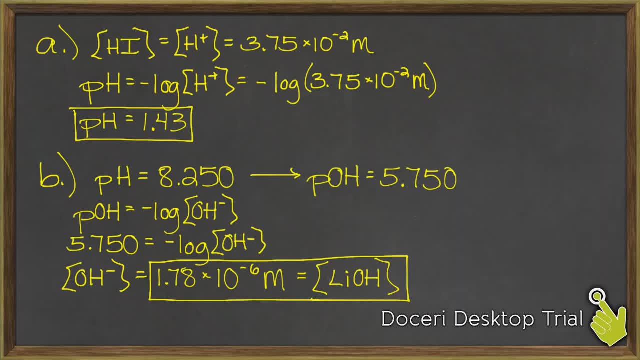 thing I did was I said: okay, well then, what's the pOH? 14 minus 8.25, and I get my pOH, which I then substituted into pOH, equals negative log of the hydroxide concentration and I was able to solve for the hydroxide ion. 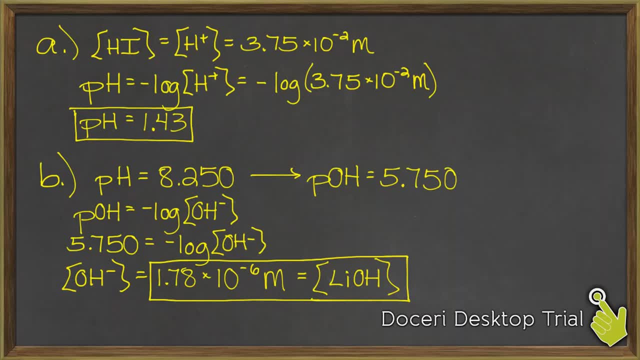 concentration And because lithium hydroxide releases just one hydroxide ion, they're in a one-to-one ratio. these two molarities are equal to one another. That would not be the case if this base was like calcium hydroxide. but since 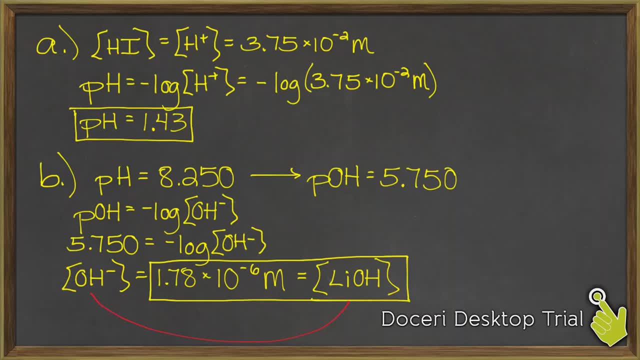 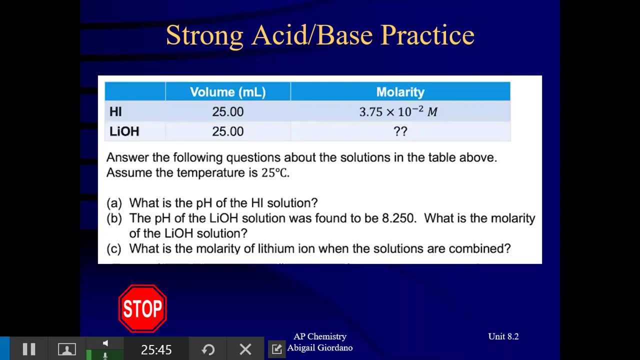 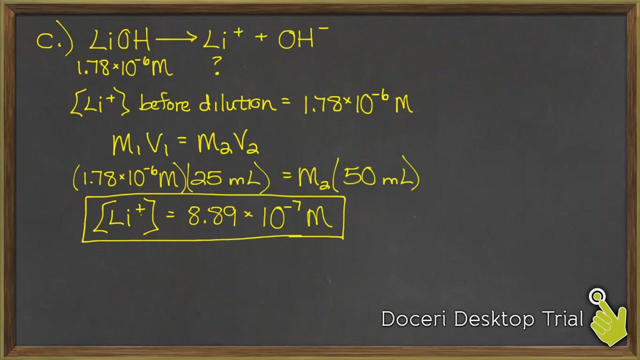 it's a base that only contains one hydroxide ion. they are, in fact, equal. Last part: we're gonna take these two solutions and we're gonna pour them together and it says: what is the molarity of the lithium ion when these solutions are combined? Okay, well, in the previous part, letter B, we just